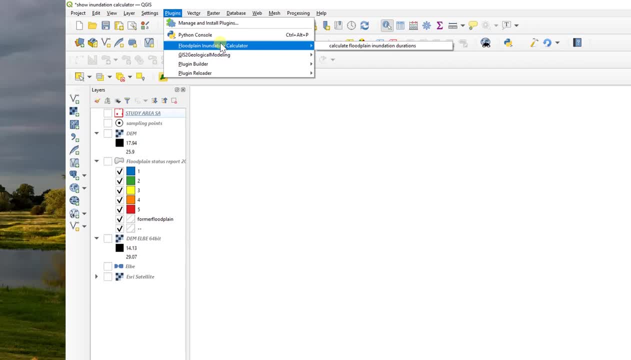 and floodplain topography. Flood duration is of great interest because it affects many ecosystem services, such as habitat provision, biodiversity, denitrification and other soil biochemical processes for maintaining water quality, and therefore we need to find simple solutions that can be applied by anyone, even if these are only rough approximations. 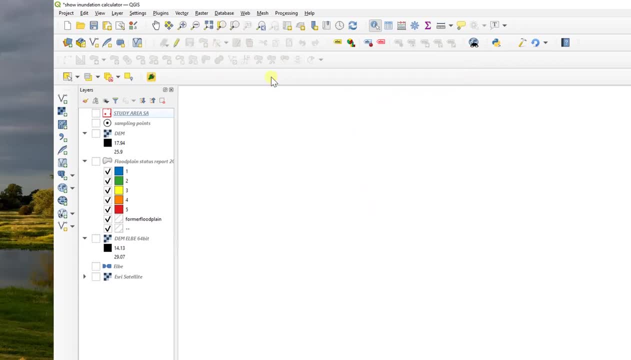 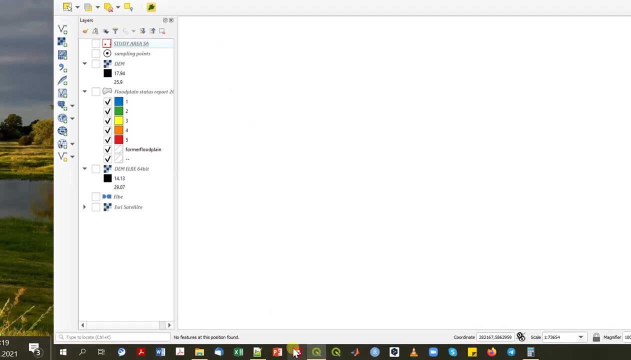 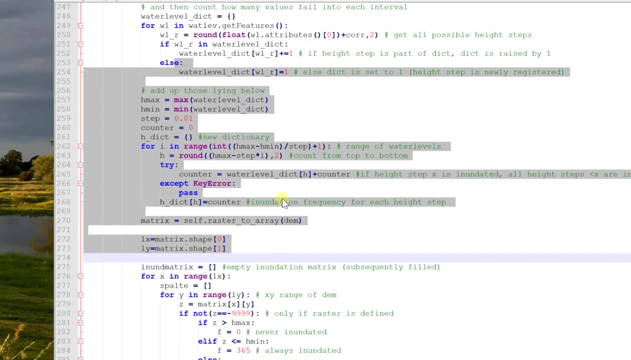 As a user of this plugin, you must be aware of the application limitations. Details of this, as well as download links for the data used, can be found in the report. I will link it below. So now some short words about the functioning of the code. Floodplain inundation is reflected. 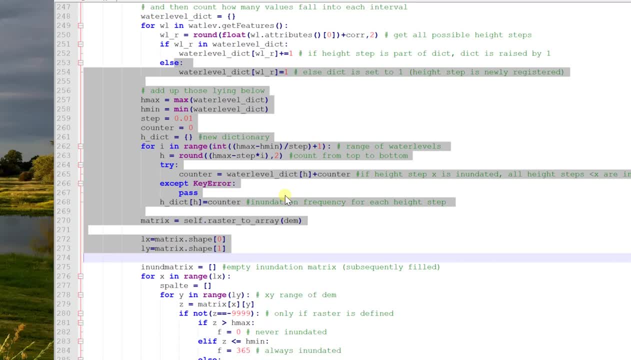 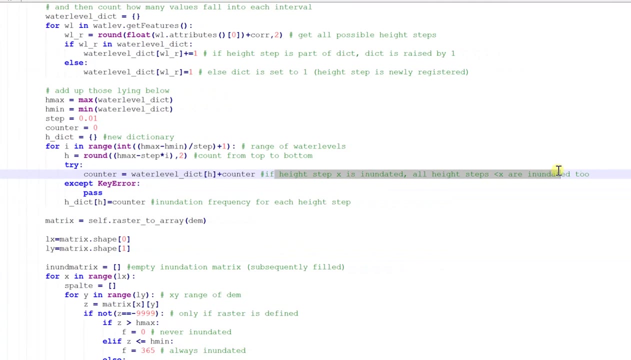 by O: A whirlwind inundation from the river channel to the floodplain when bankfull conditions are exceeded, and flooding from below ground through the filling of the level of aquifer. Based on this raster, cells with an elevation below the current river water level are assumed. 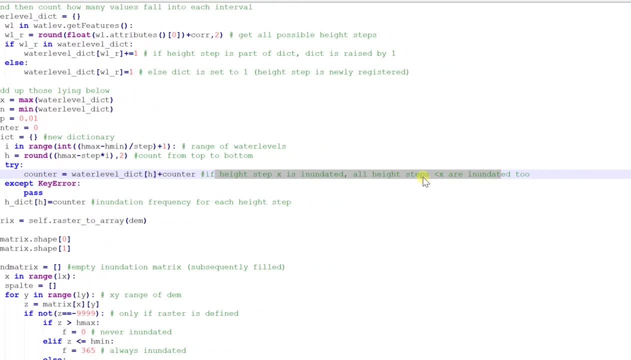 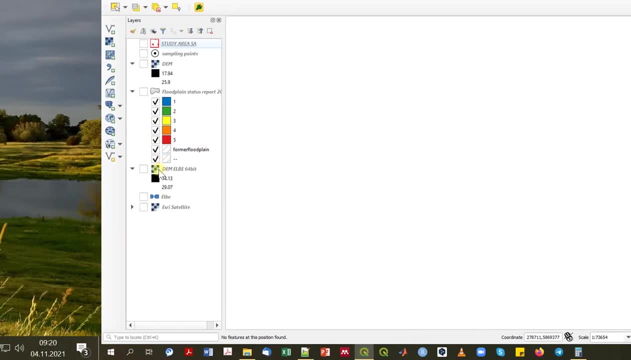 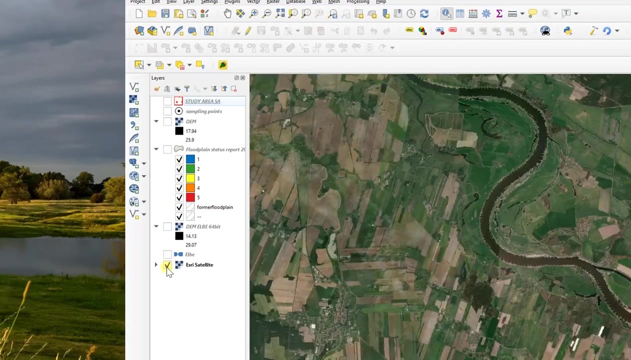 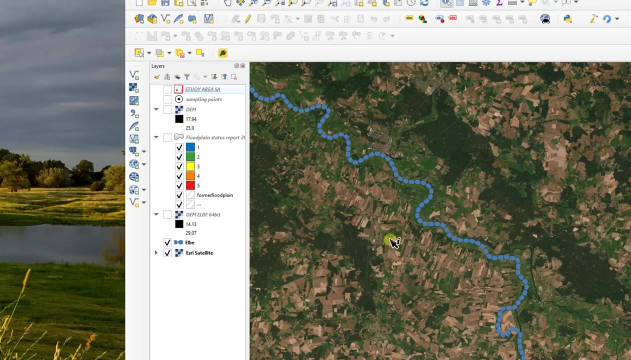 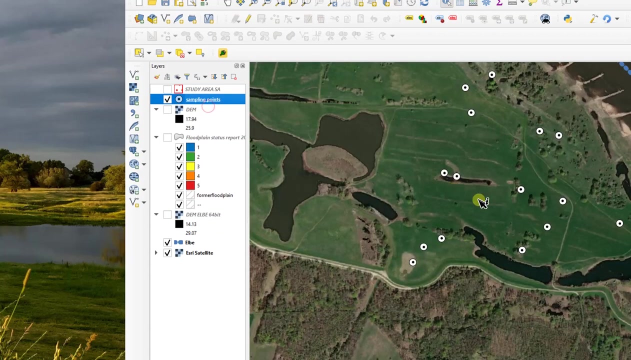 to be inundated in the modeling process. I would like to show it using an example along the Elbe river. So here we go. This is a satellite image of a part of Germany. This is the Elbe river. I have some sampling points over here. Let's zoom to the layer so you can see it better. 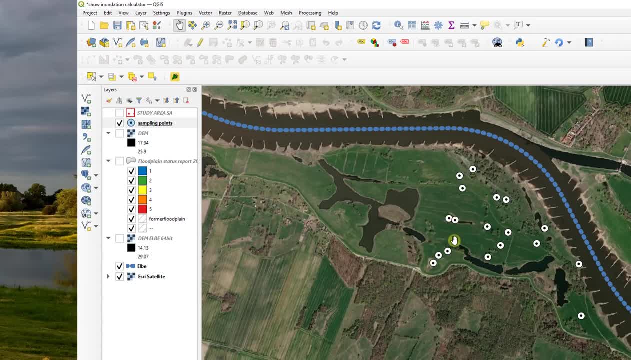 I would like to know how many days these points- or let's say, any point in this area. I would like to know how many days these points are In this case. I would like to see how much of this level is flooded. I would like to know how much to see here. 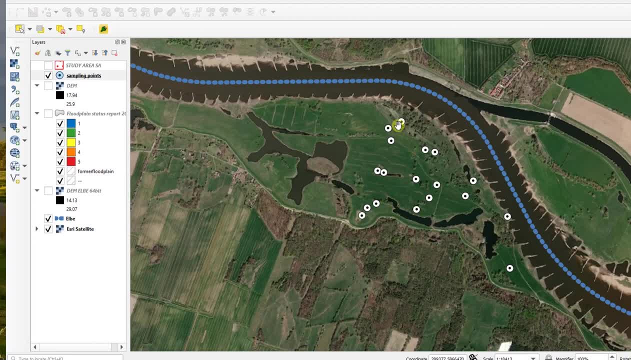 Let's see if this is a flat surface here, And if it is still a flat surface, what will happen. So the average level of this kind of river flow is flooded on average per year. So first I need a polygon, for which I would like to have this information. 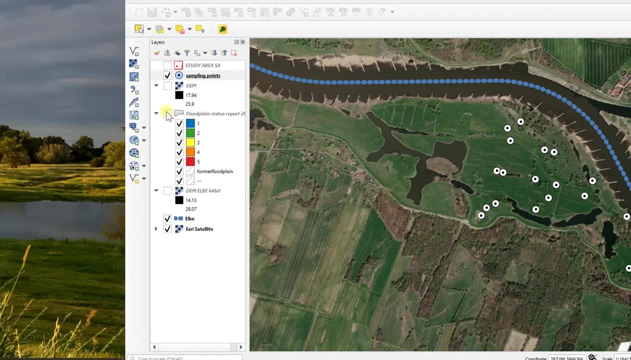 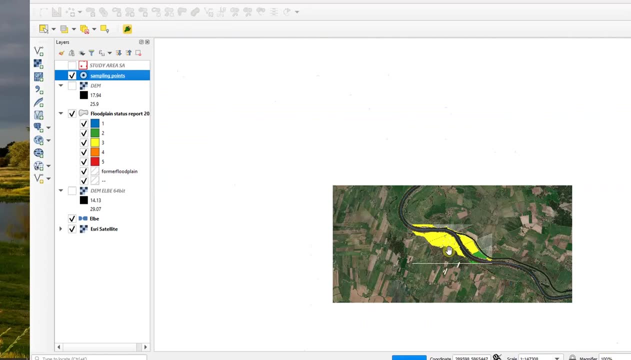 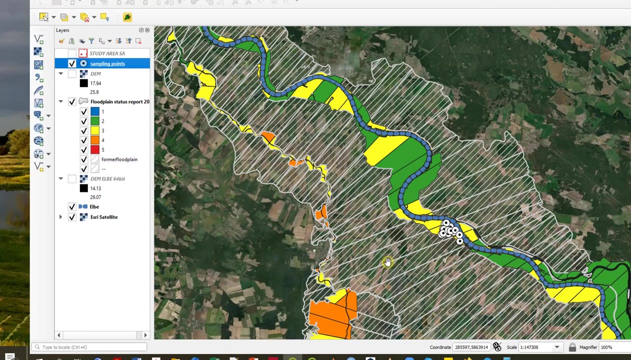 For German rivers. you can use the floodplain sections Which were assessed through the state of support in German floodplains. You can access them using the web feature service provided by the federal agency of nature conservation. For detailed information, you can have a look at the video above. 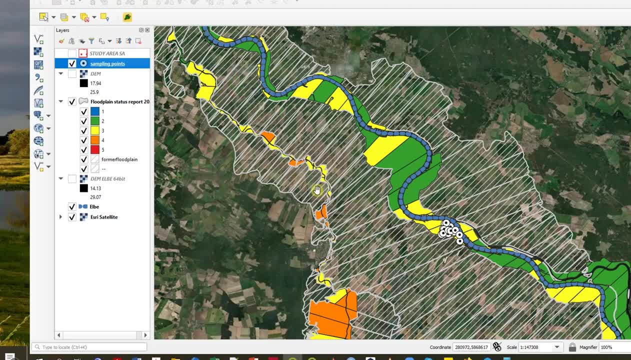 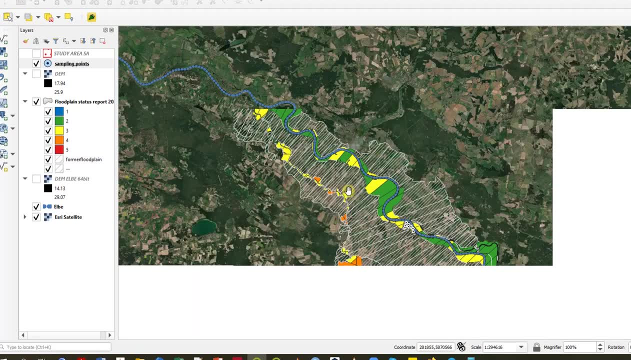 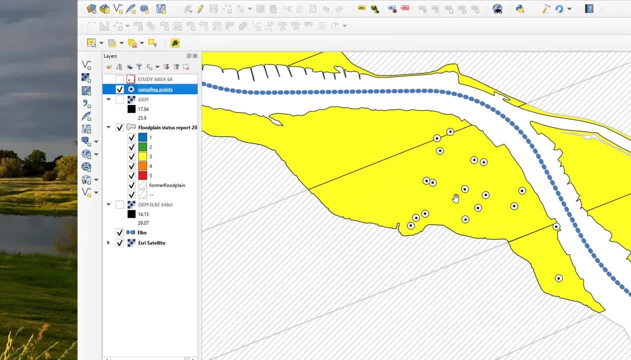 Please go to the website and try this feature. If you are interested in this kind of feature, please apply this feature and update your data. a look at the report link below and you can see the colored parts show the active floodplain and the striped area is the former floodplain. So my sampling points are located in three. 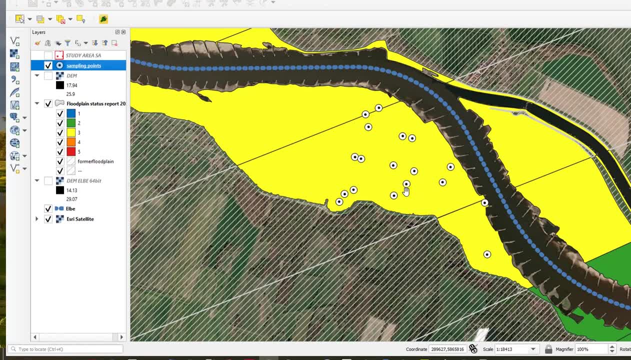 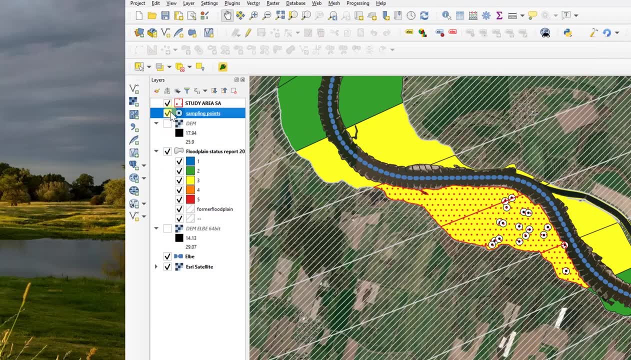 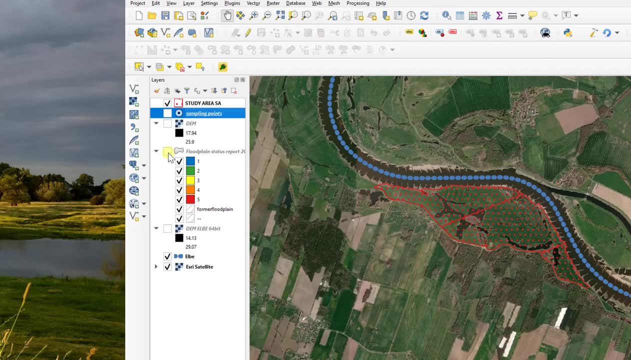 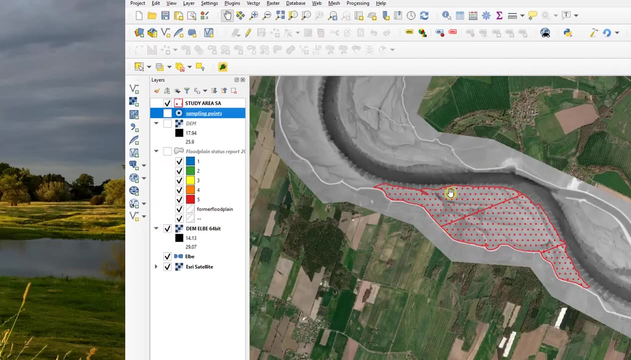 of this active floodplain sections, So I clip my study area to that size. Next, I need the digital elevation model for my study area as a 64 bit tiff. This is the digital elevation model of the Elbe floodplain. and again, which can? this can be found online too. and again, I clipped it to the size of my study area, like this: 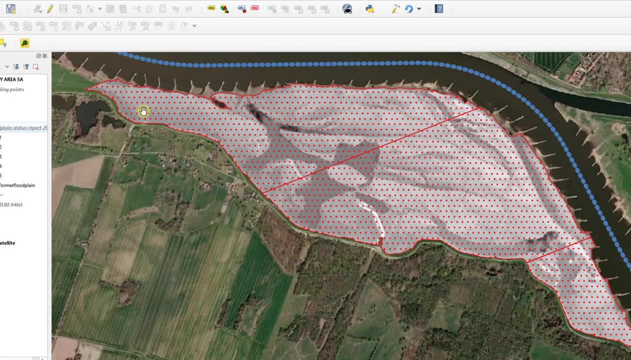 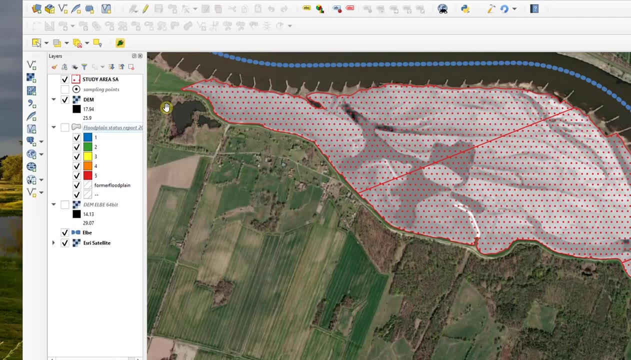 So now I need the daily water level information. I need one value per day and the same unit as the digital elevation model, so meters above sea level. Yeah, you might get them upon request, and please provide the daily water levels in one column of a csv file. 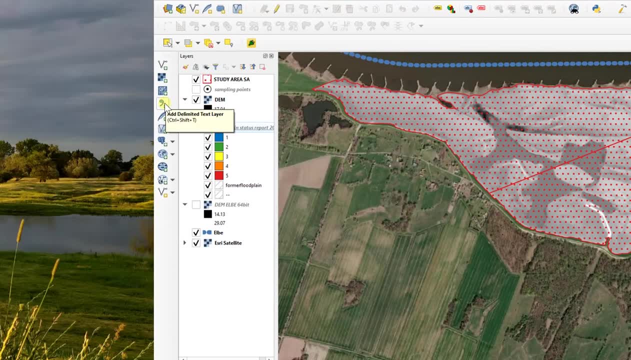 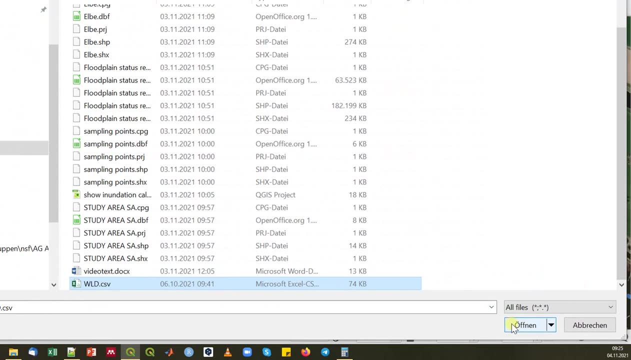 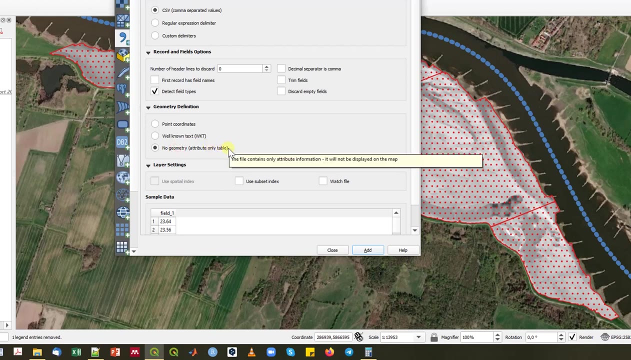 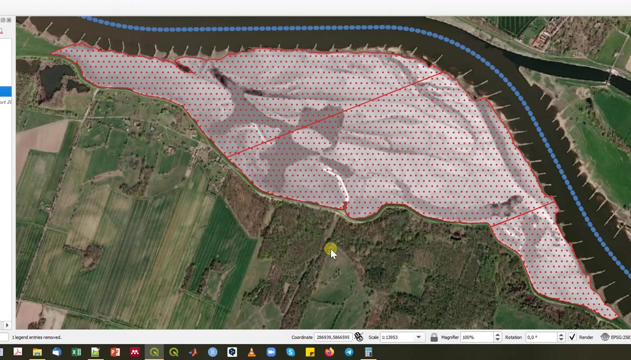 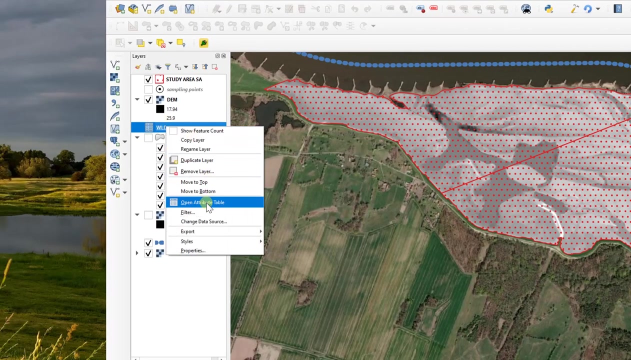 So let's add this one. Add delimited text. choose your file with the water level data, open, click on no geometry attribute, only table, and check the preview to make sure everything is correct and add. Now the table appears as a csv file in the layer list and by opening 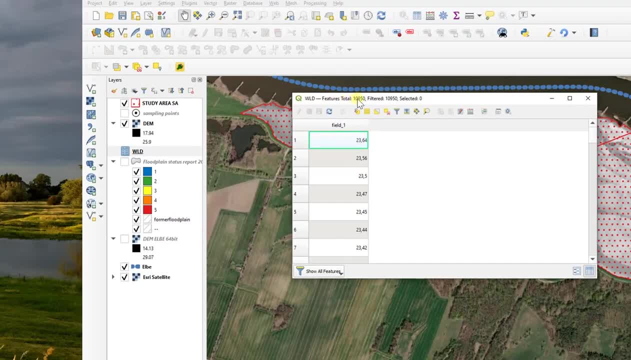 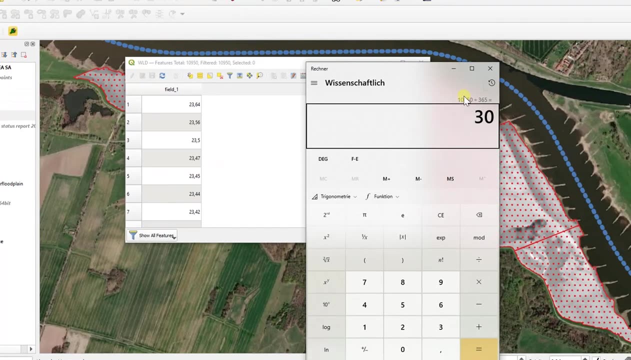 the attribute table you can check the total features. Make sure that the column length is a multiple of 365.. So in my case, I have 10 950 water levels and 10 950 divided by 365.. In my case, I have 10 950 water levels and 10 950 divided by 365. 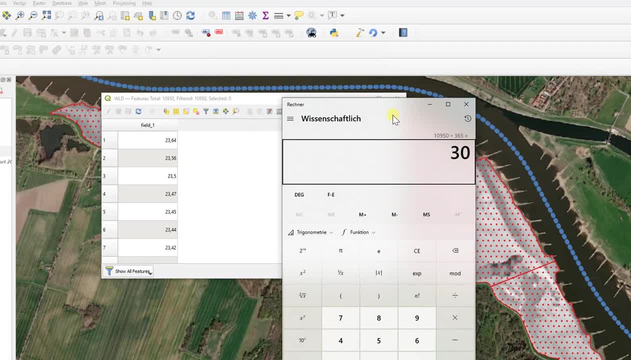 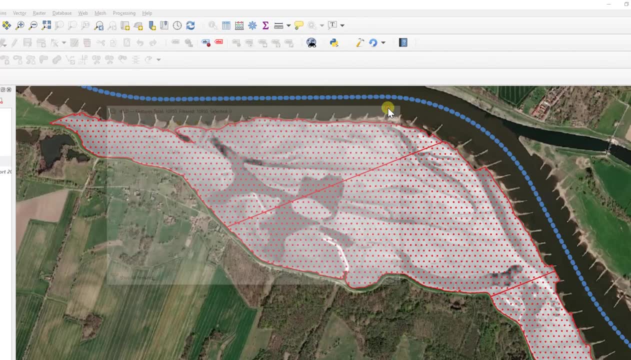 I need the precise values to give me an accurate estimate of the volume. So in my case I have 10 950 water levels, and 10 950 divided by 365. means 30, so 30 years of water level data. Okay, if the gauging station is not. 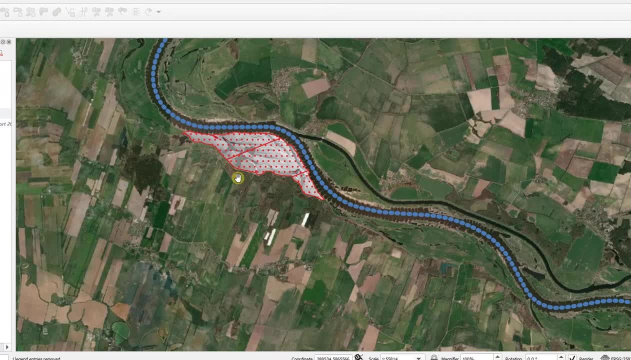 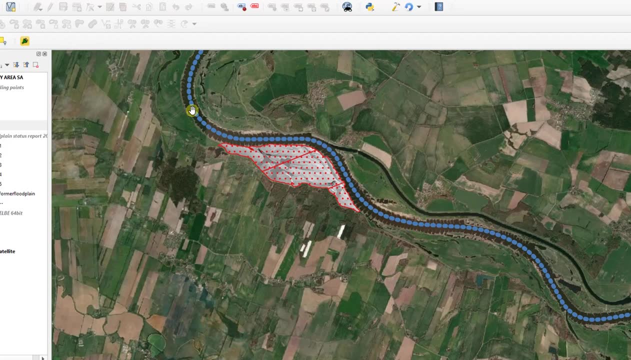 directly located next to the study area. you can make at least one real-time water level difference measurement between the water level at the gauge and the water level in the study area, which for sure is also a rough approximation. but you can input the difference as correction factor X. So okay, now we have. 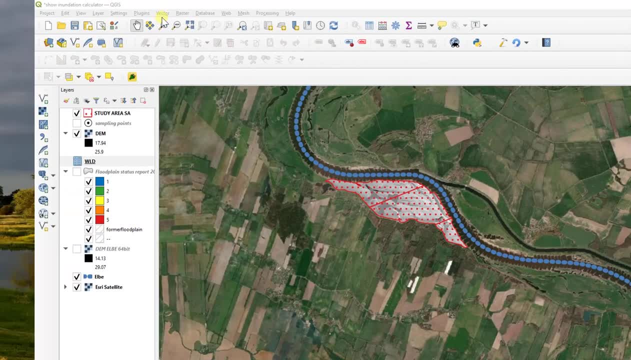 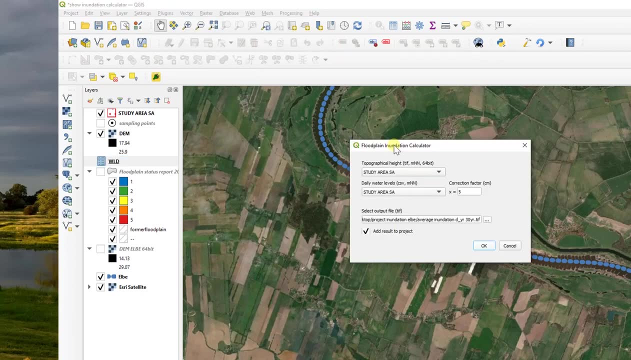 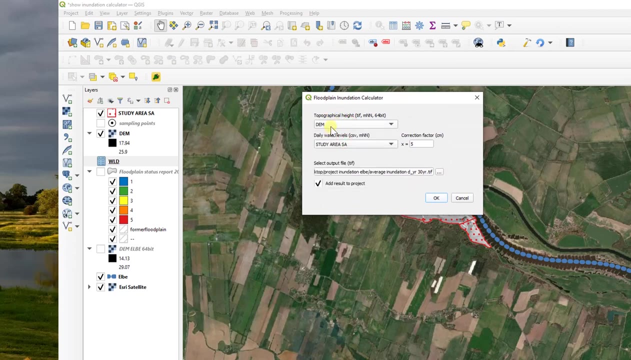 prepared all of our data, let's start the plug-in. Plug-in flat-plane inundation calculator: calculate flat-plane inundations. The user interface asks for the topographical height, so the DEM, which was clipped to the size of our study area, and the daily water levels, so water level data and the. 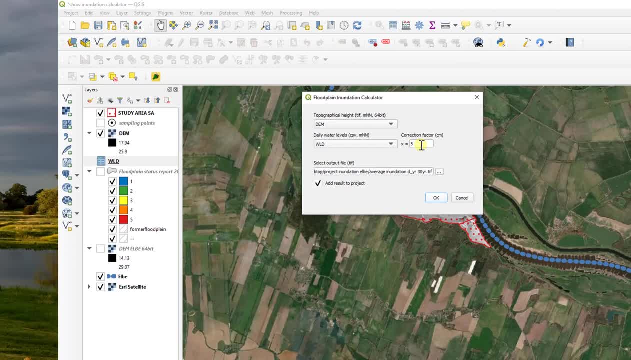 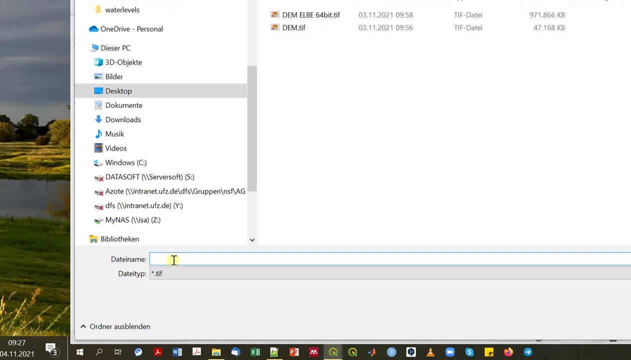 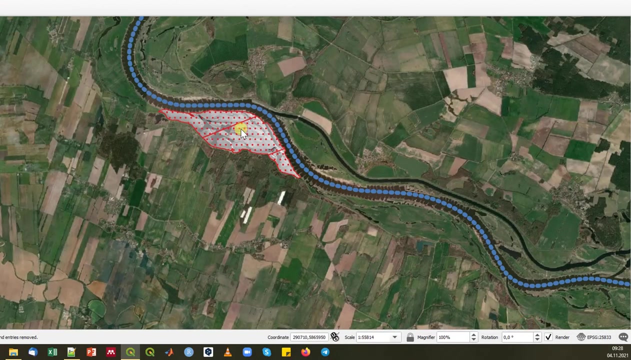 correction factor, which in this case is only 5 cm because the gauge is closed, And finally select the output file by specifying a path. So I recommend to include the considered years and a filename, so average inundation days per year, 30 years basis or something like that, and save Okay and that's it. It's. 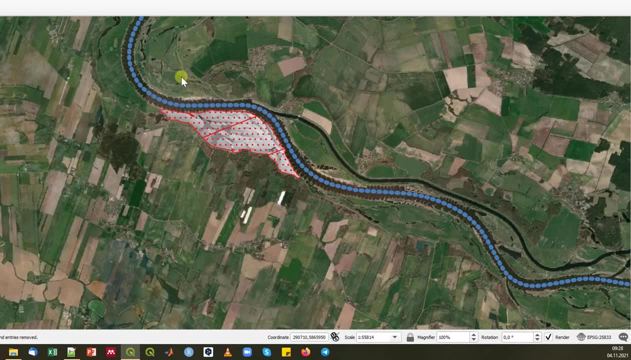 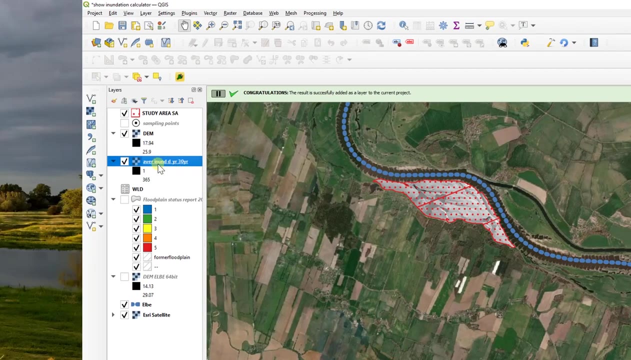 very simple, isn't it? And, yeah, now we have to wait a little bit and, if everything went well, you will see a congratulation message and a new layer will appear in the layer list. Congratulations, And this is our new. 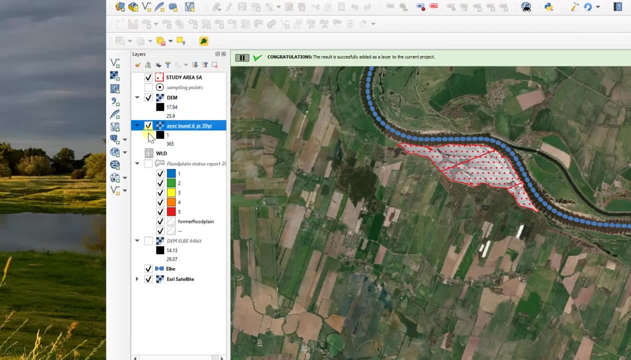 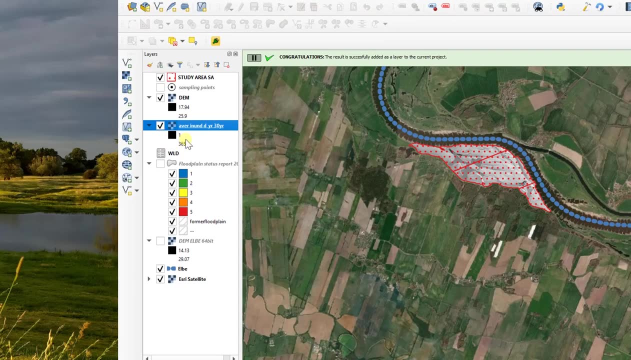 layer. The new layer contains values in the range of 0 to 365, or narrower. and yeah, the standard topology is a black-to-white gradient, but for a nice visualization I recommend plotting average inundation days per years in quantiles. 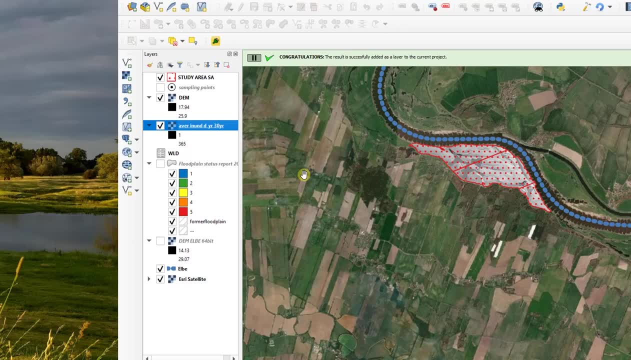 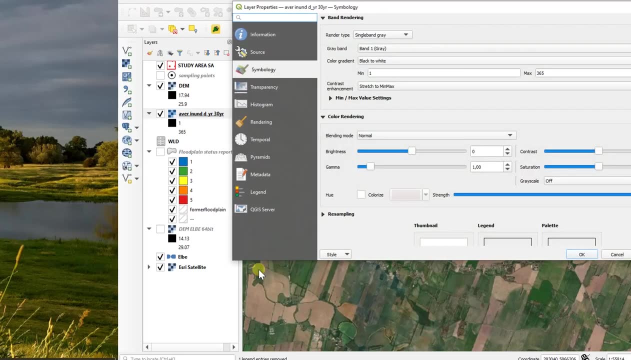 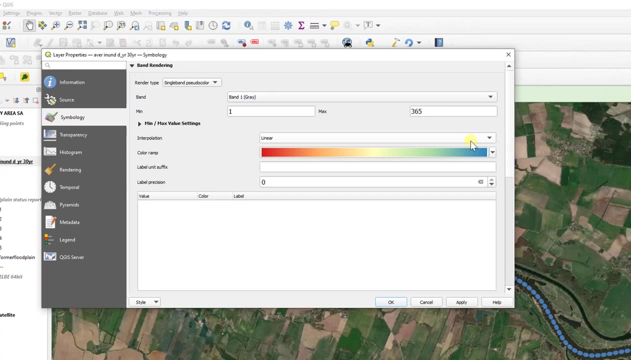 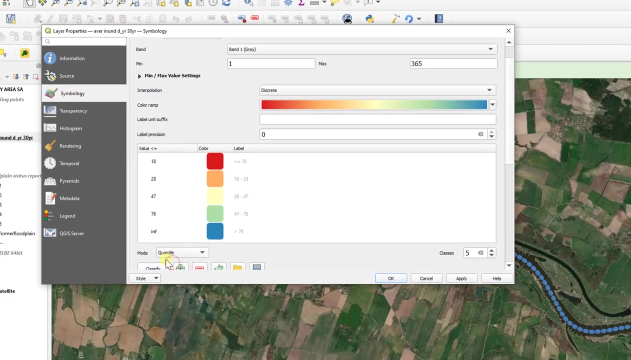 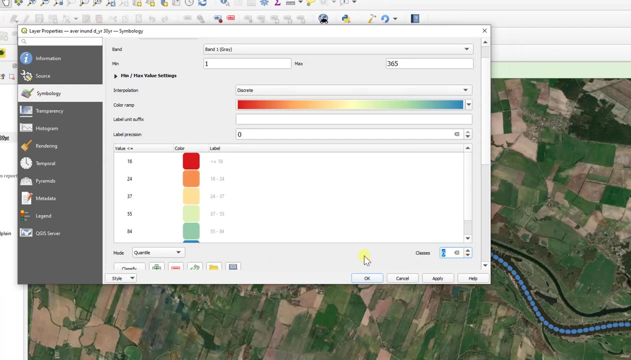 By this the entire area is divided into equally sized classes. So right-click on Properties, Symbology, Render Type: Single Band, Pseudocolor Interpolation in Discrete Equal, in Quantile Mode, Quantile, and choose 5 classes or 6 classes or whatever.